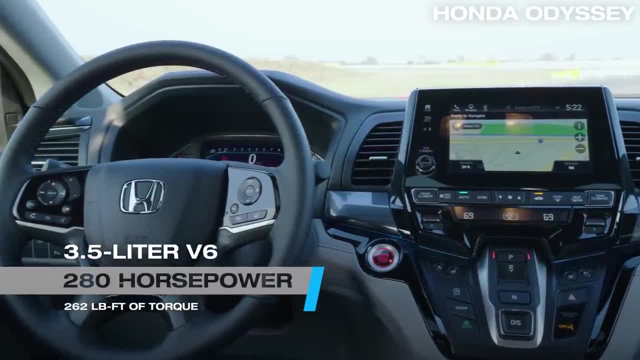 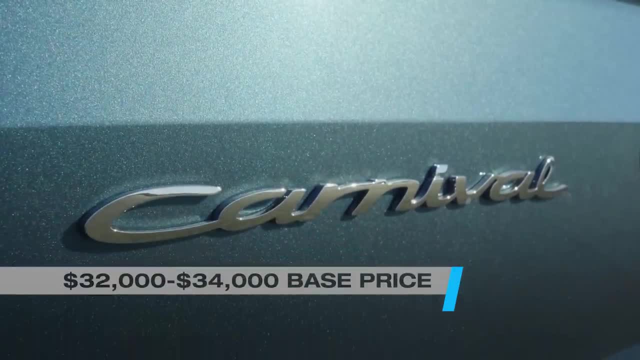 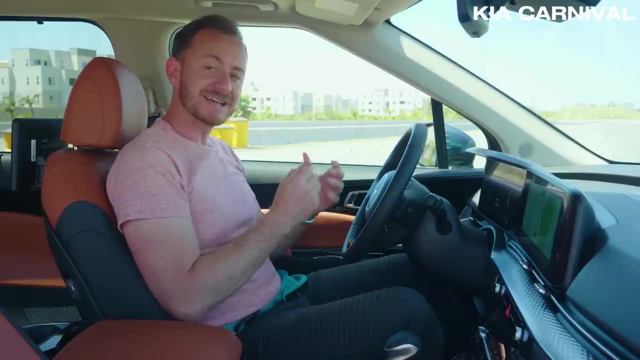 enjoyable to drive and it's packed with modern safety and tech features. Each of these starts around $32,000 to $34,000, but you should expect to pay about $40,000 for the most popular trims and options. So what stands out inside the Carnival? Well, you get excellent materials and 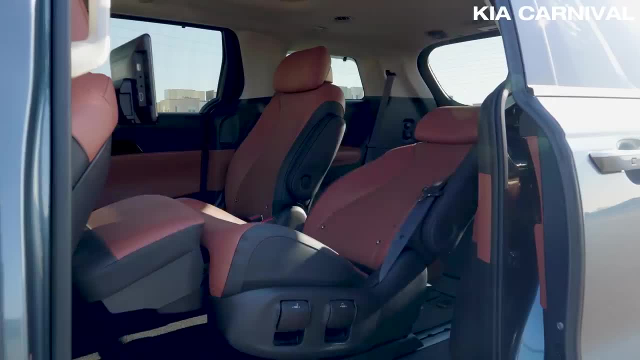 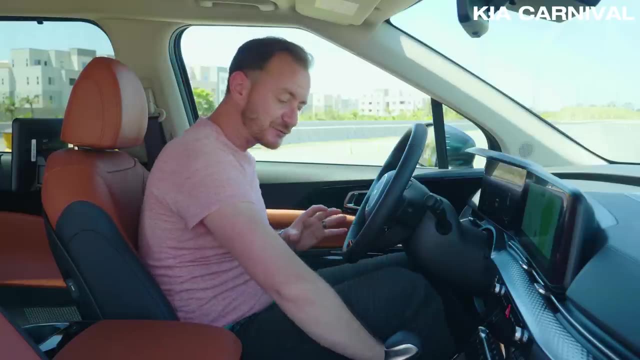 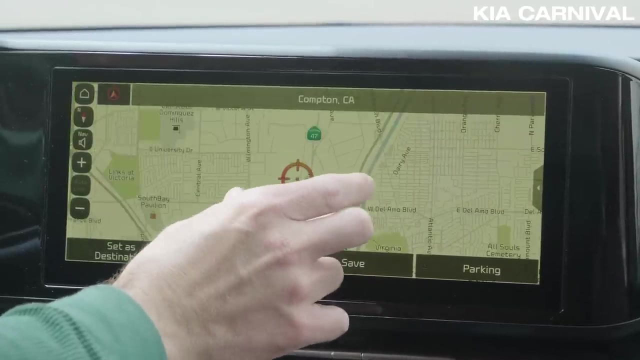 pretty comfortable seats on this SX Prestige trim. There's also lots of interesting textures and soft surfaces throughout the interior. It's kind of a bummer that there's no pass-through storage under here, like on some of the other minivans that we have, but you get huge, vibrant screens with menus that are easy to control. 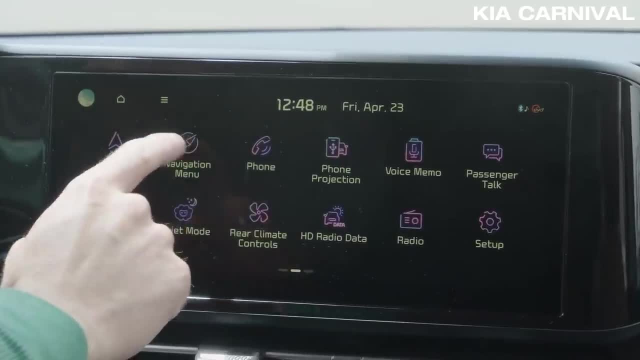 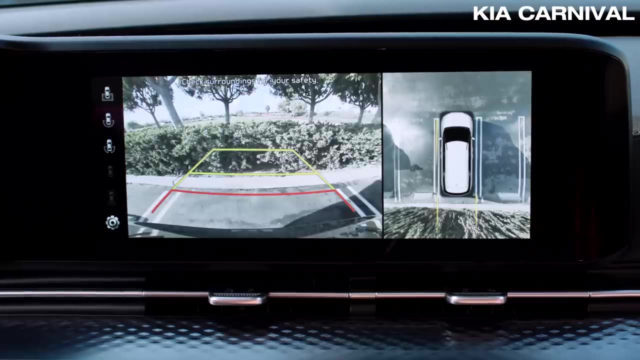 using all of these buttons, although I wish they were a little bit bigger. You also get wireless, Apple CarPlay and Android Auto. The large screen is perfect for seeing the bird's eye view to make parking a breeze. Unfortunately, the piano black. 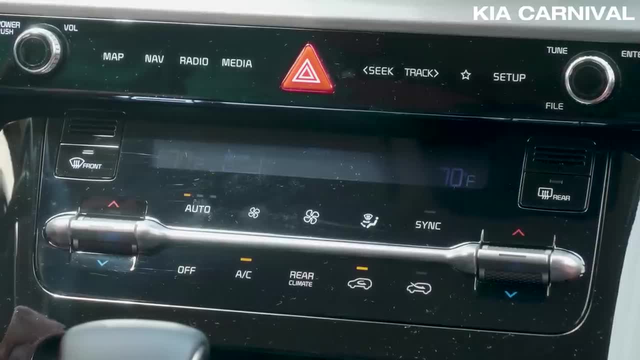 soft and light-colored screen on the SX Prestige trim is a little bit too big for the driver. The soft touch buttons below it smudge easily and they don't have haptic feedback. Lastly, we wish Kia's smart trunk feature activated more predictably. 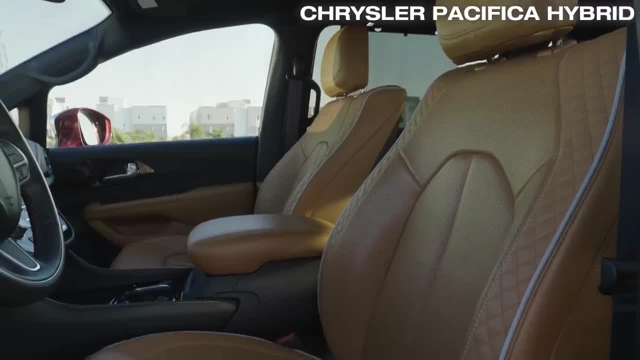 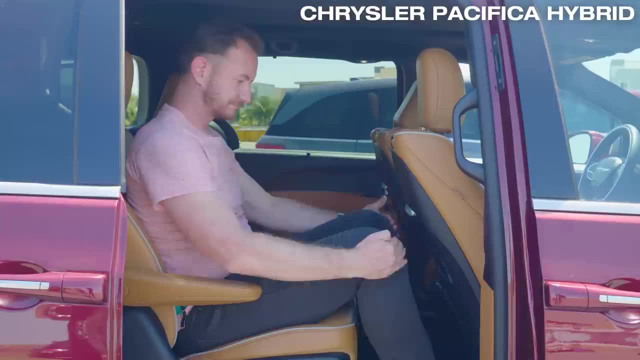 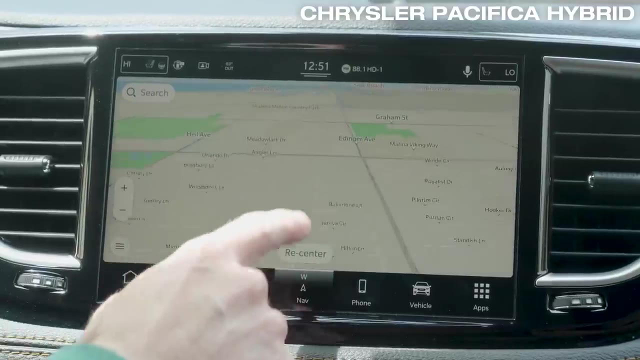 In the Pacifica there's a new top trim called the Pinnacle, with quilted leather seats and pillows. There's huge sliding doors and easy access to the third row Leg room is just about average, though. Its Uconnect infotainment system has clear graphics, quick responses and good native apps. 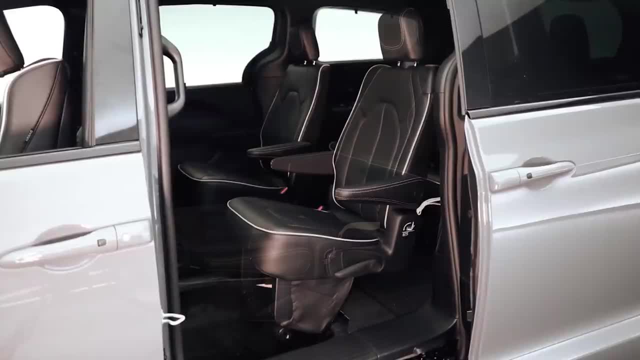 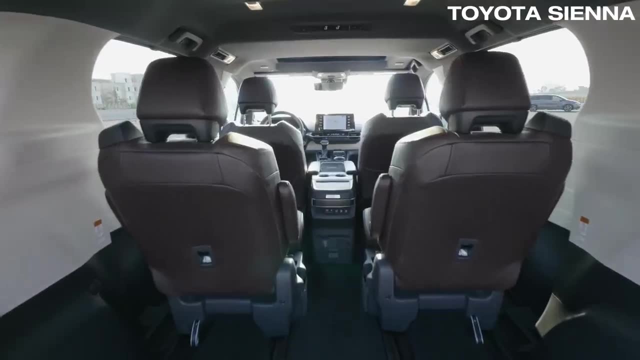 Unfortunately, the hybrid battery means you don't get the stow-and-go feature that lets you fold rear seats into the floor. In the Sienna it's easy to get in and out thanks to good interior packaging and large door openings. There's also a large central touchscreen, but it glares in. 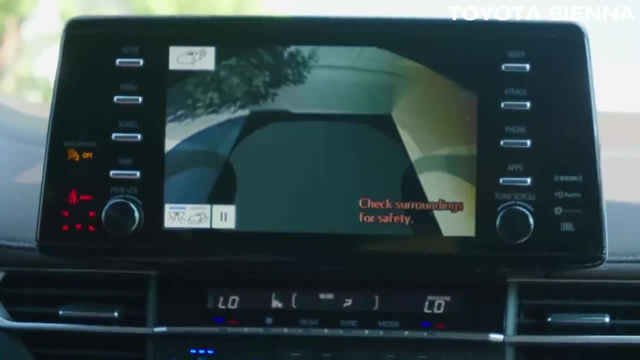 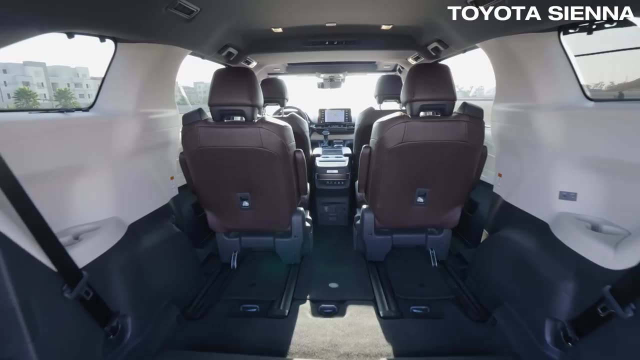 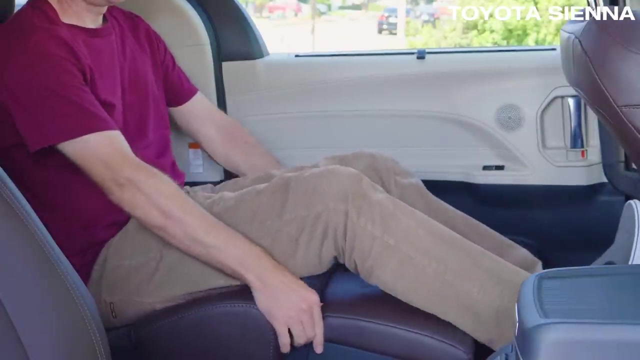 direct sunlight. Thankfully, there's a digital surround view camera and a digital rear view mirror available, if you want. The in-cabin fridge and vacuum cleaner that we love so much is discontinued for 2022 due to supply. Now the second-row seats slide the farthest and have the most leg room, but due to the integrated 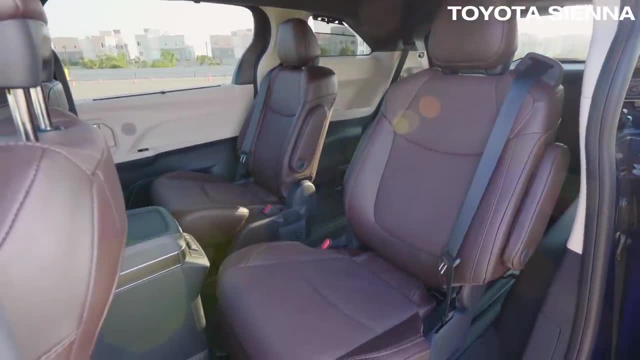 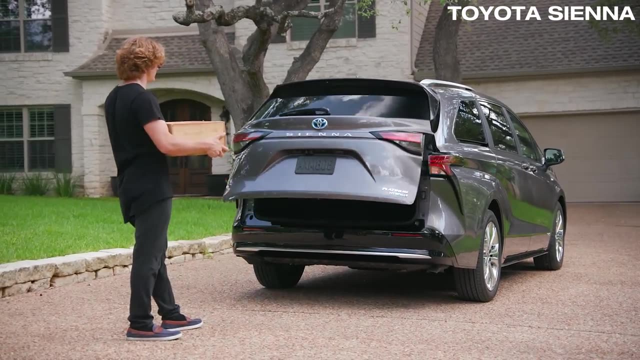 airbags. you can't take them out. This is the only van in the class that you can't remove the second-row seats on. We have mixed feelings about the kick-open side doors and rear hatch, because sometimes they work and sometimes they don't. In the Odyssey, the second-row seats are at just the 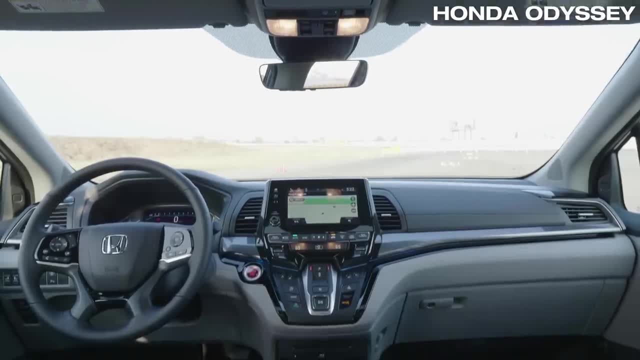 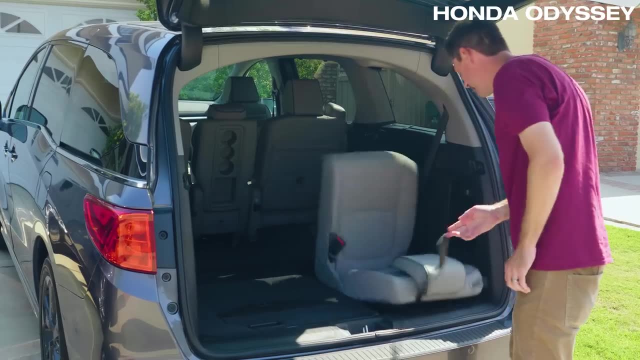 right height and they also recline As the driver. you get so-so visibility over the hood and pretty bulky pillars. There's also no surround view, which is a good thing. In the Sienna there's no surround view when you're backing up. It has stowable rear seats, but the in-cabin vacuum cleaner is. 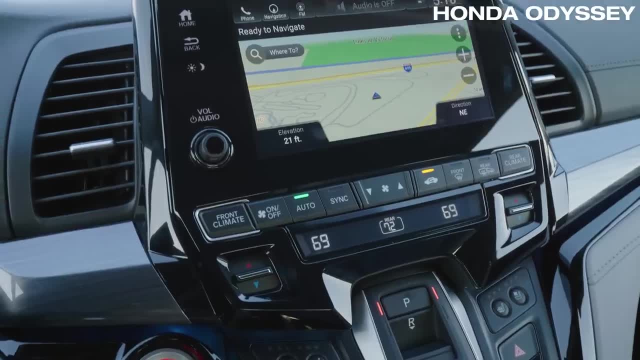 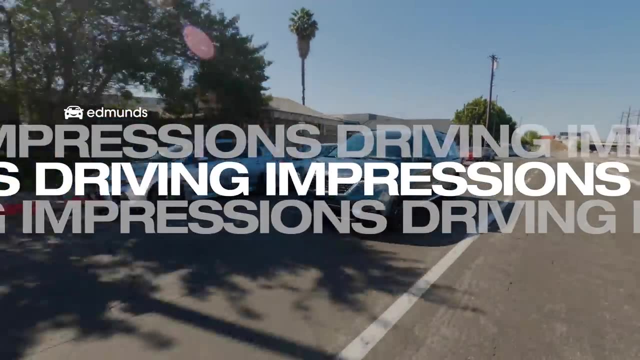 discontinued, at least for this year, due to supplier issues And the infotainment system feels dated. Now that we know a bit about our magnificent minivans, let's see how they drive on the road. All right behind the wheel of the Kia Carnival. As we said, the Carnival is powered. 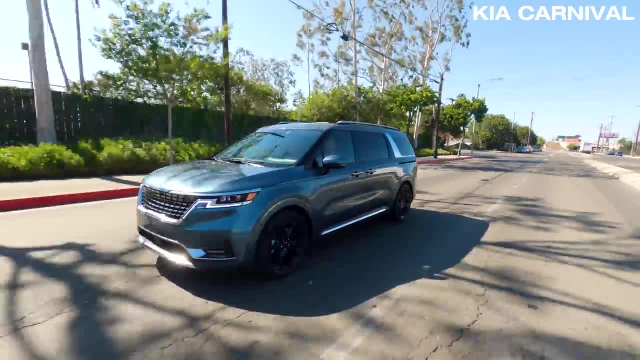 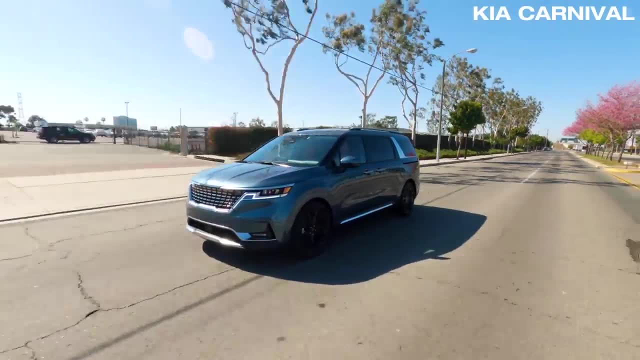 by a V6 engine and it feels plenty strong for this vehicle. There are no issues with feeling underpowered or getting off the line too slow, anything like that, In fact. it's got a lot of power. If you step on it, the transmission will downshift pretty quickly and it'll even give you. 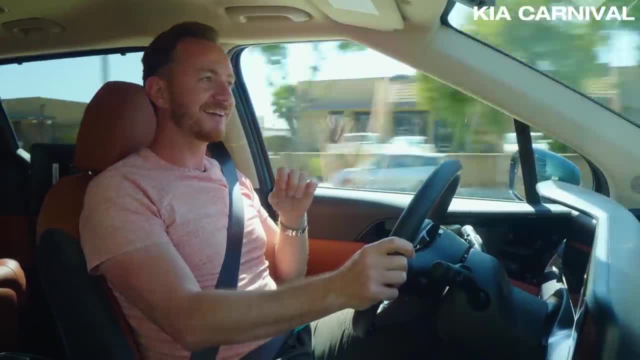 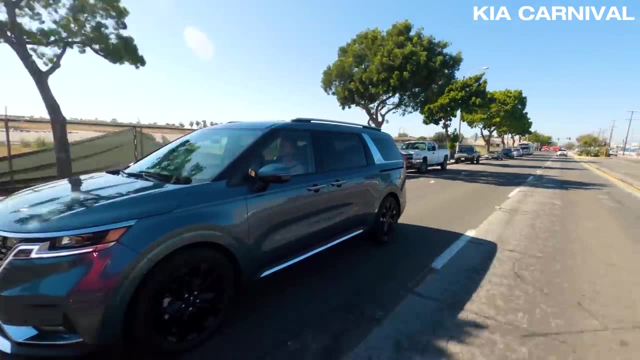 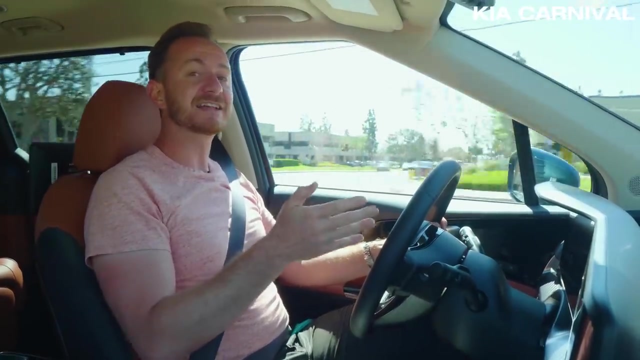 a little bit of a roar Hear that Under the hood. all good marks for the Carnival. It also delivers a nice, smooth ride. To be fair, the suspension is a little bit more firm in the Carnival than some of our other minivans, And when it comes to steering and handling, this feels more like. an SUV, whereas some of those other vehicles really do mimic how it feels to drive a smaller car. When it comes to fuel economy, the Carnival is EPA rated at 22 MPG combined, which is right in line with other front-wheel drive minivans in the class. However, its highway rating is down 2 MPG. 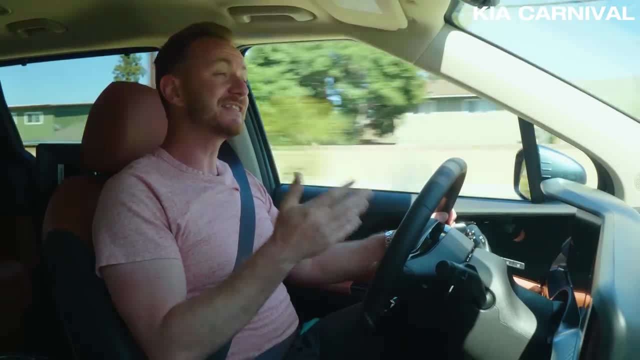 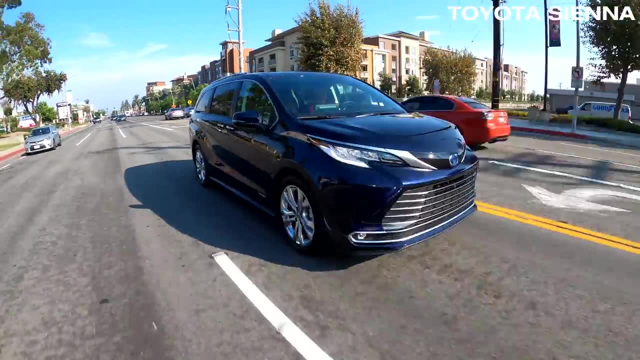 compared to the Odyssey and the Pacifica. And if you're really that concerned about fuel economy, you should probably be looking real hard at the Sienna Sienna time. The Toyota minivan is smooth but ultra slow. Its brakes are also a little tricky. 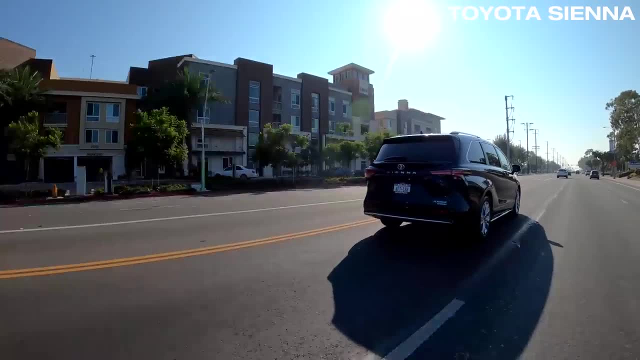 to use, sometimes Not quite as smooth as the Sienna, but it's still a good car to drive. Not quite as smooth as the Sienna, but it's still a good car to drive. Not quite as smooth as the Sienna, but it's still a good car to drive. Not quite as consistent as the other competitors here. 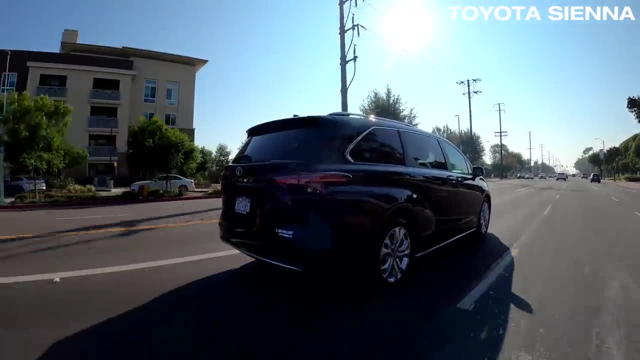 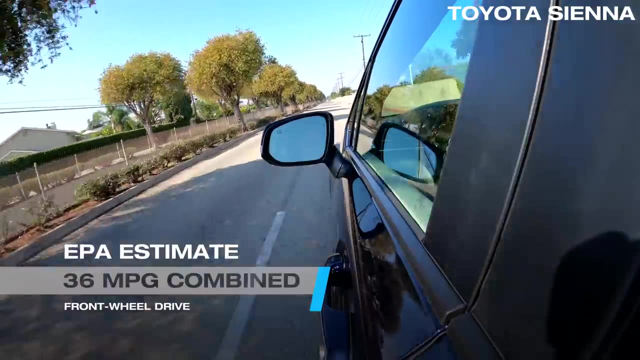 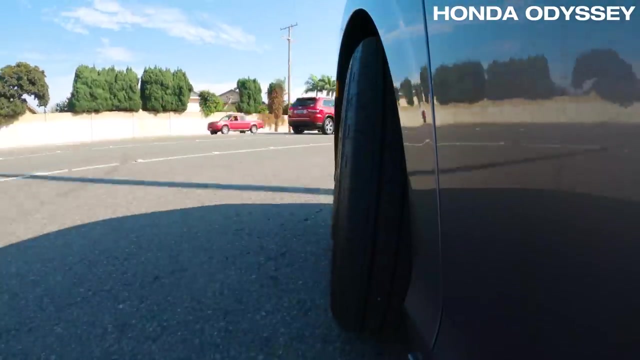 But the steering is light and easy, which is great when you're tooling around the Gymboree parking lot. On the plus side, it's EPA rated at 36 MPG. combined Fuel economy is exceptional. Believe it or not, the Odyssey is borderline fun to drive, with precise steering and braking. 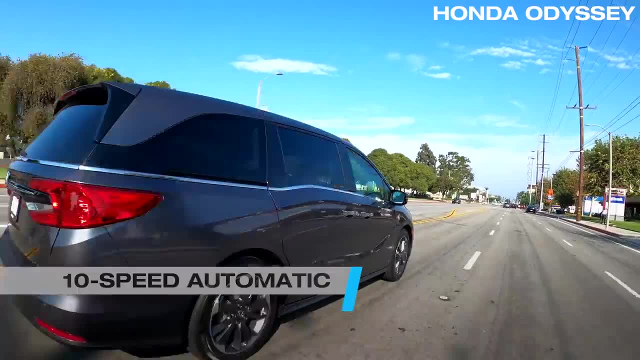 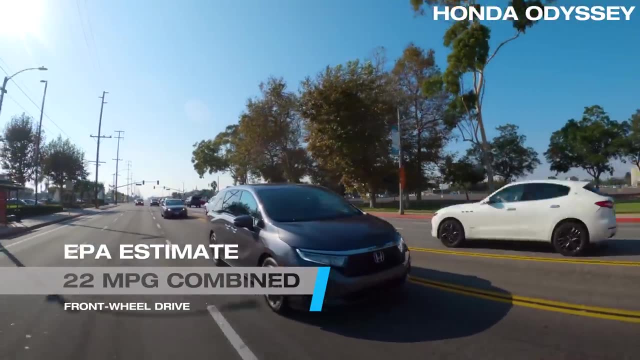 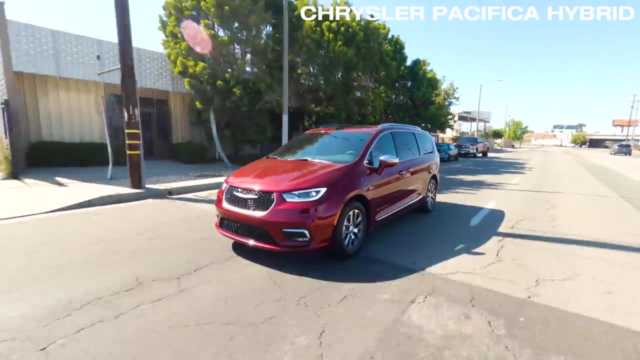 It all just feels cohesive and well put together. Even the 10-speed automatic transmission is sorted out nicely. Its EPA rating is 22 MPG, which is true of all Odysseys, because there's no all-wheel drive or hybrid version, When in EV mode this Pacifica plug-in hybrid offers instant torque that moves the van sharply.